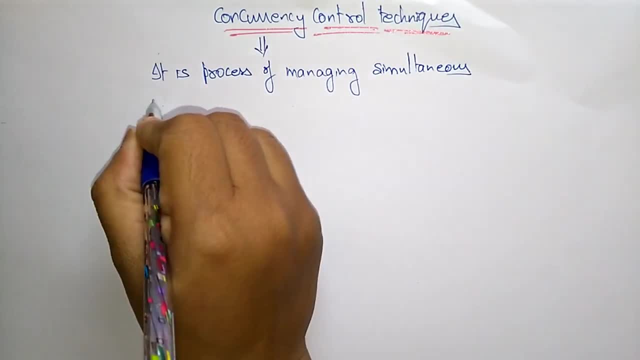 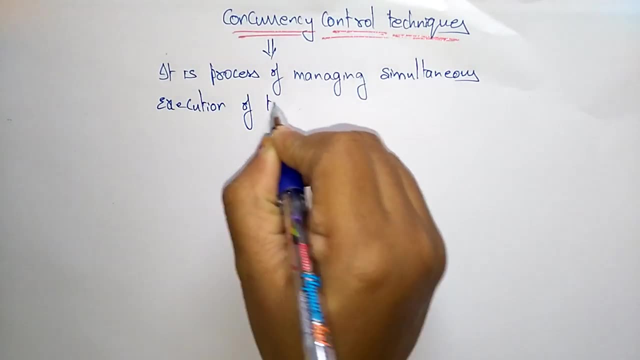 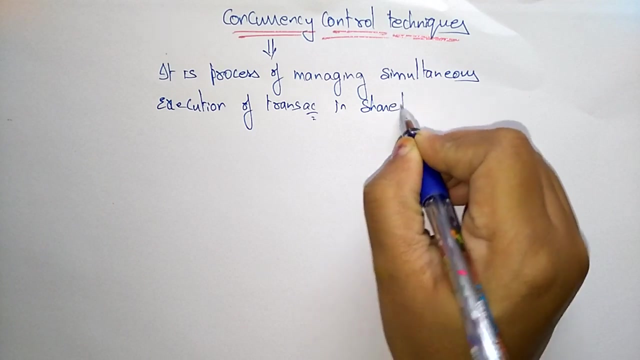 simultaneous execution of transactions. Simultaneous execution of transactions- So if you take so many transactions, is the concurrency- is a process of managing all the simultaneous execution of transaction in a shared database. So the main thing is in a shared database. Suppose if all of the people are using so many. 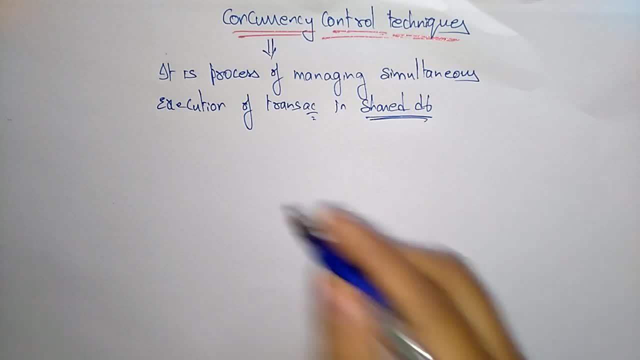 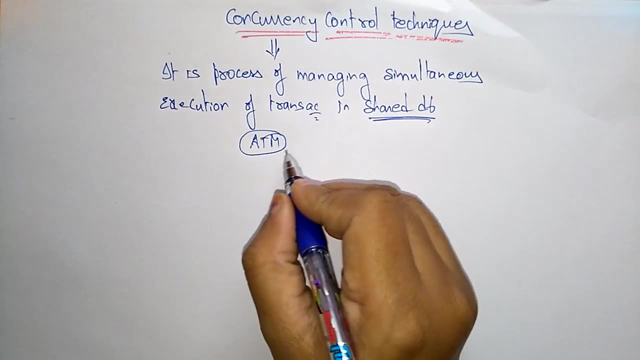 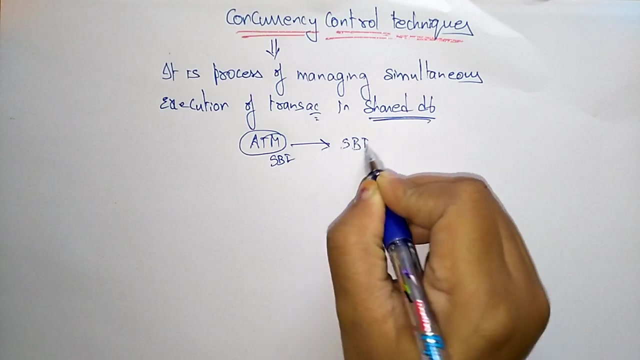 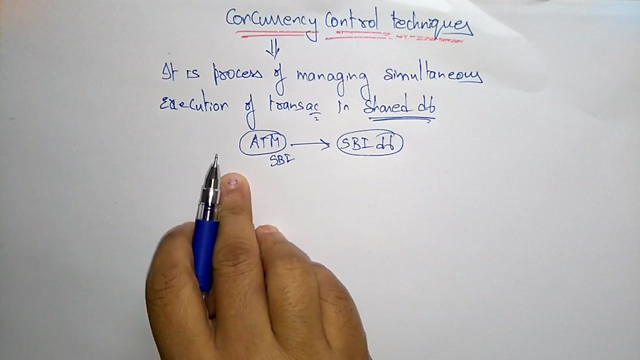 of people are using the same same database. Suppose ATM. I already said this example. So different people are accessing the same ATM, the SBI ATM. This is SBI database. So all the people, so many people, are withdrawing their money by using the ATM. that is SBI ATM means they are interacting with the SBI database. 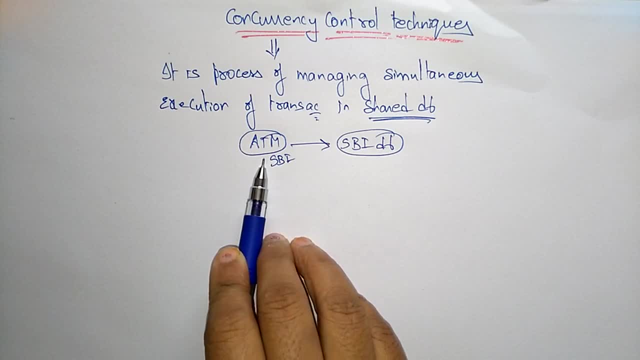 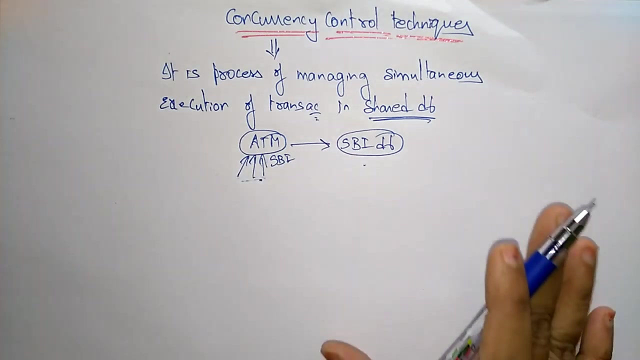 So here so many transactions or multiple transactions are done on the same database. So this you call it as a concurrency. So concurrency is a process of managing simultaneous execution of transactions So different people are accessing at the same time. So this concurrency is managing all the simultaneous execution of these transactions who are working on the same database. So that is, they are sharing the database. That you call it as a concurrency technique. Sorry, concurrency control. 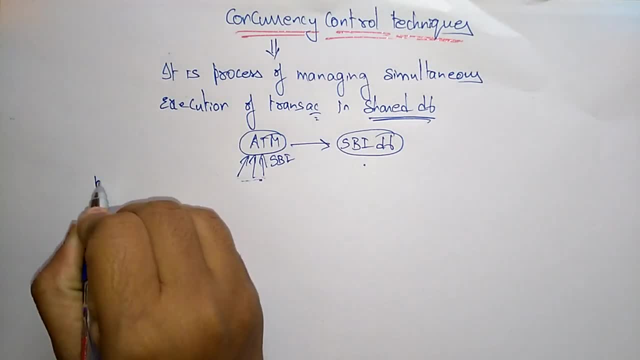 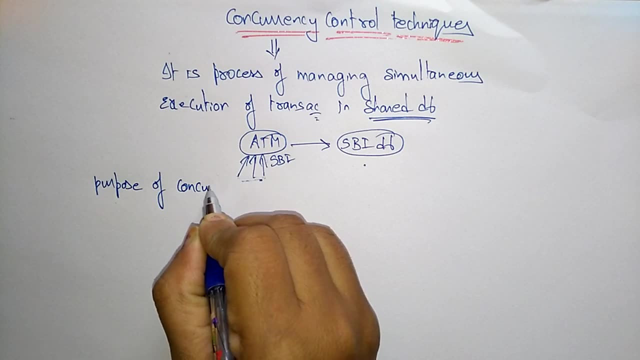 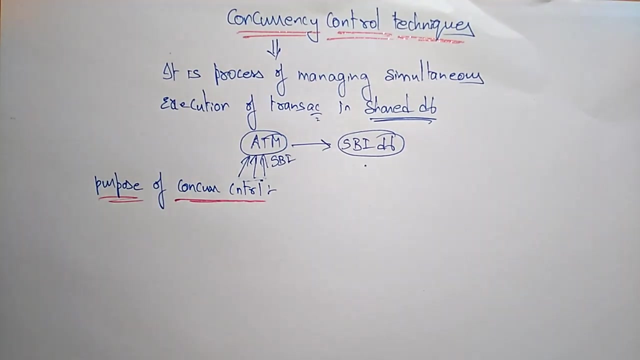 So let us see what are the purpose of concurrency controls, Why we are using this concurrency control. Purpose of concurrency control: Okay, So what are these purpose? So the different purpose of concurrency control is: first, one is to ensure, to enforce, to enforce isolation. So everyone knows that whatever the database that should be accessing or the transactions that are accessing on the database should be in isolation. So the purpose of using the concurrency control to enforce them into isolation. 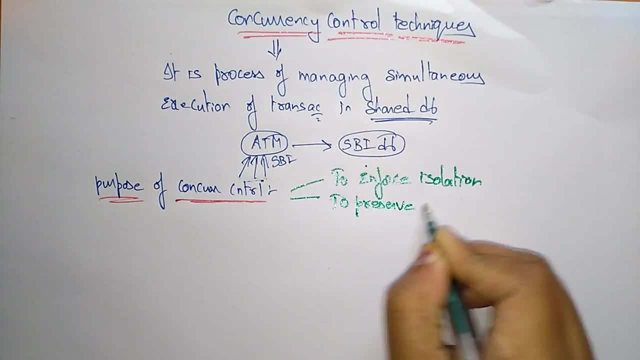 To preserve database consistency- So you are maintaining the database always in consistent state- And to resolve conflicts. So, and this concurrency control is used to resolve the conflicts. What are those conflicts? Read-write conflict, write-read conflict and write-write conflict. So I already discussed this in the previous video. Okay, 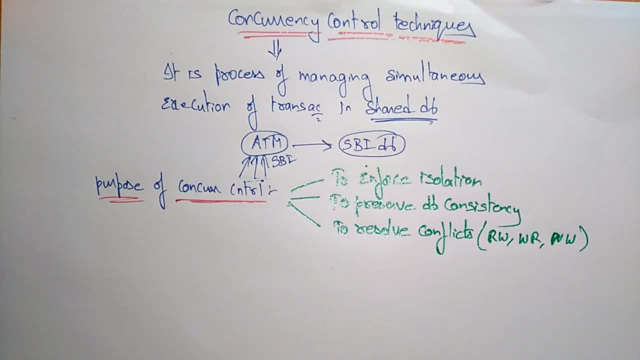 So the purpose of concurrency control is: we are using this concurrency control to enforce isolation, to preserve database consistency and to resolve the conflicts of read-write, write-read and write-write conflicts. Okay, So this is the purpose. So let us see what are the techniques that are techniques of concurrency control. So to maintain a concurrency, and you have to maintain it- 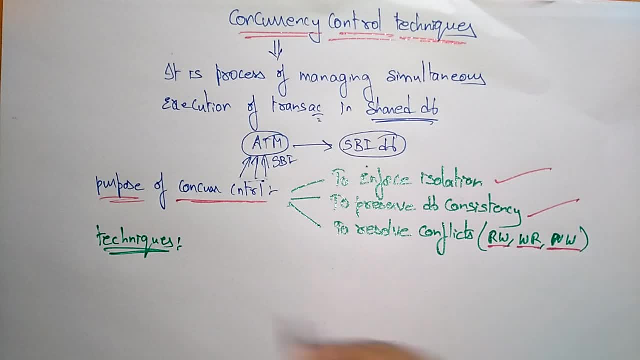 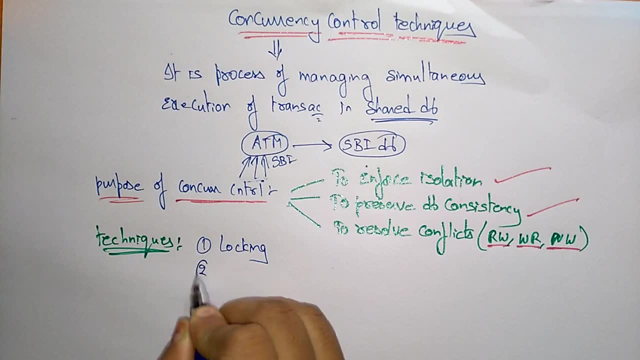 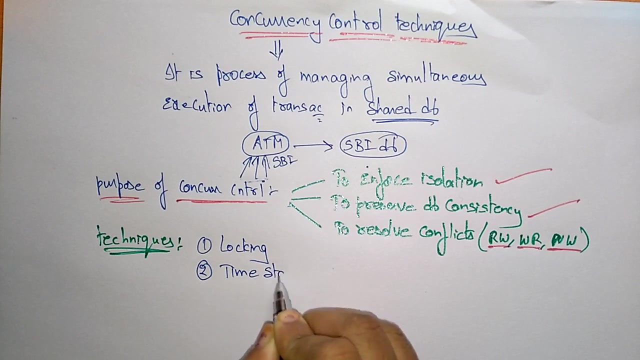 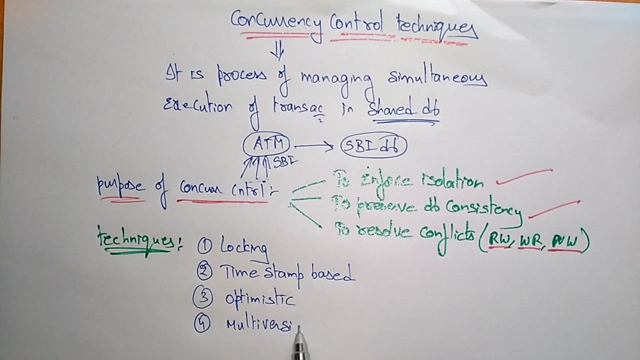 So what are the techniques that are involved? or first one is locking. Locking is one of the technique used in the concurrency control: Timestamp based, Timestamp based. Third one, Optimistic. And fourth one is Multiversion. So these are the four techniques that are used in the concurrency control: Locking, Timestamp based, Optimistic And multiversion. Okay, So let us see the first technique: Lock based protocol Locking. So what is this locking? 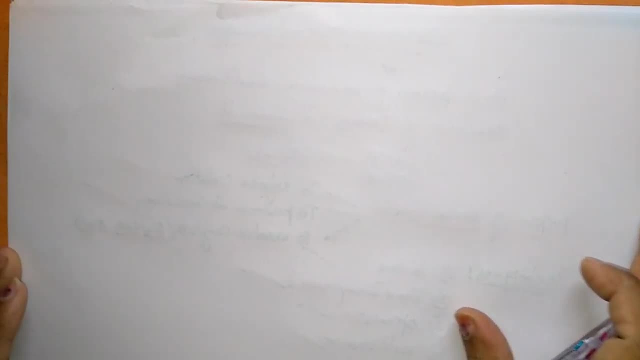 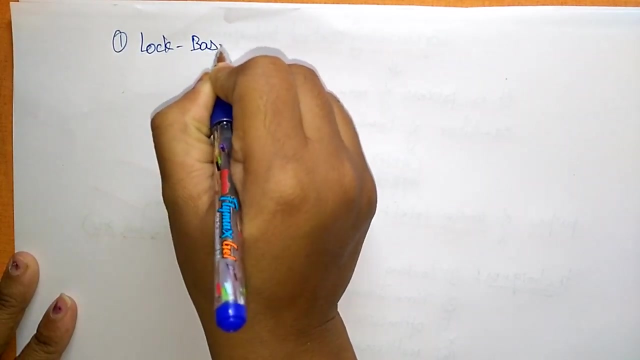 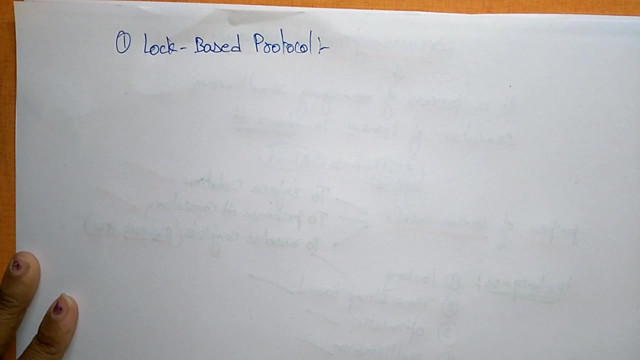 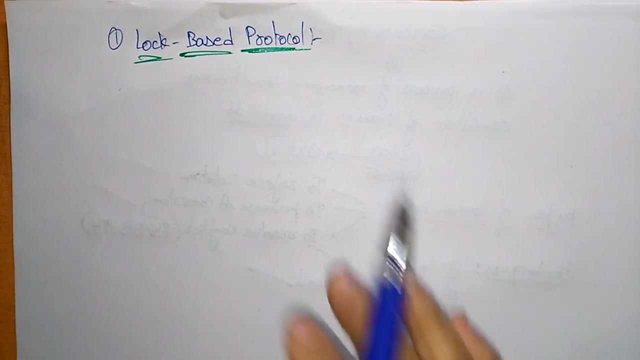 So the first technique in concurrency control is Lock based Protocol. Okay, So what is this lock based protocol? The name itself is saying It is locking the transaction. So, whatever the transaction it is doing, It first locking the transaction, Doing the operations Again, after that it releasing the transaction lock By using unlock. Okay, So a lock. 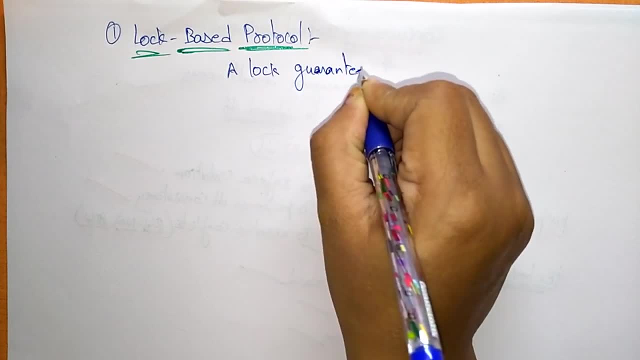 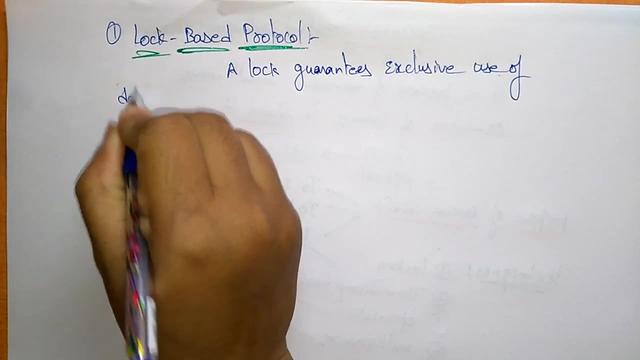 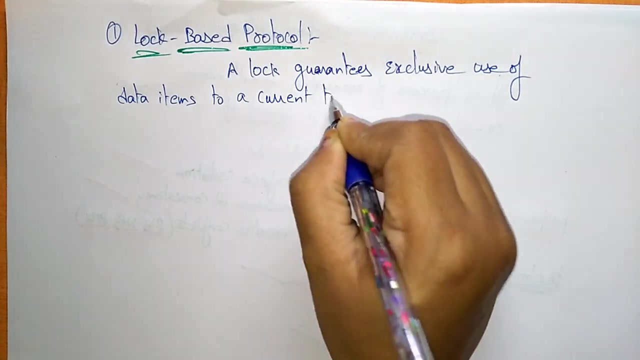 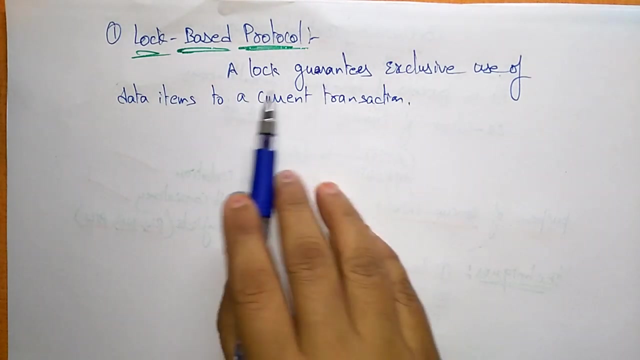 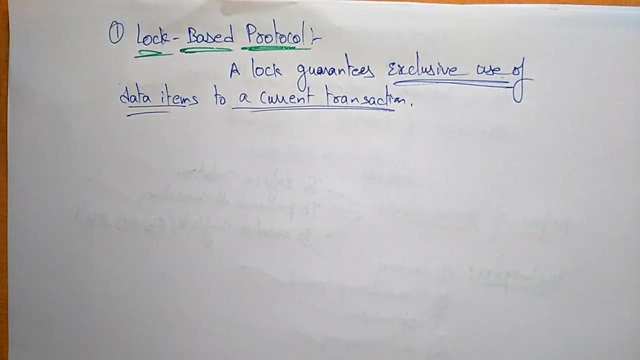 Congressional Sidewalk- Exclusive use of Data Items. Exclusive use of data items to a Current transaction. So that is a purpose of using the lock, So the lock based protocol. Here the lock guarantees what it ensures: the exclusive use Of transaction. So if the current some particular transaction is executing, so those data items will. 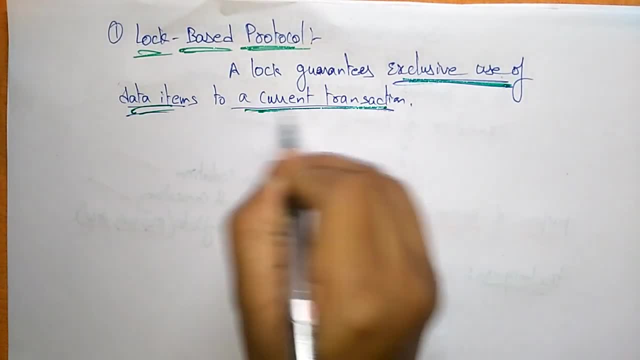 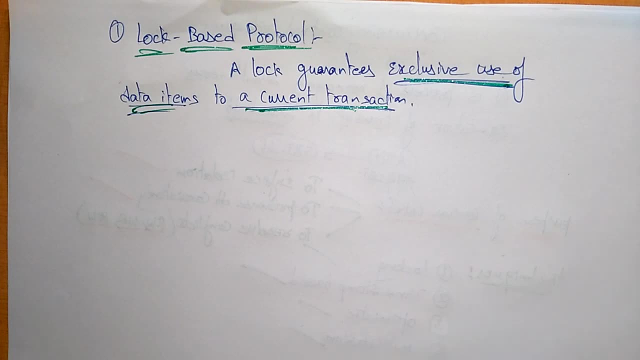 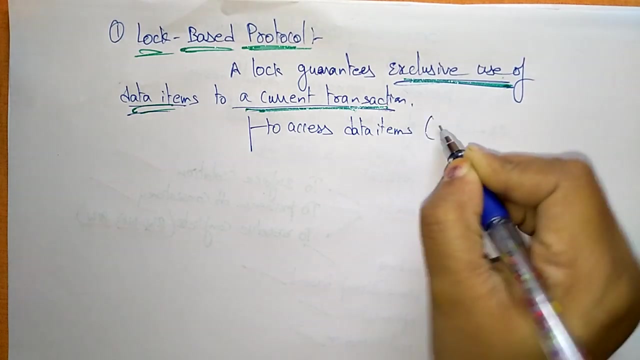 be exclusively used for, only for the current transactions. For that purpose we are using the lock. So this lock ensures the exclusive use of data items to a current transaction. So what it does first, it access the access data items. So, whatever the how it access the data items by lock. 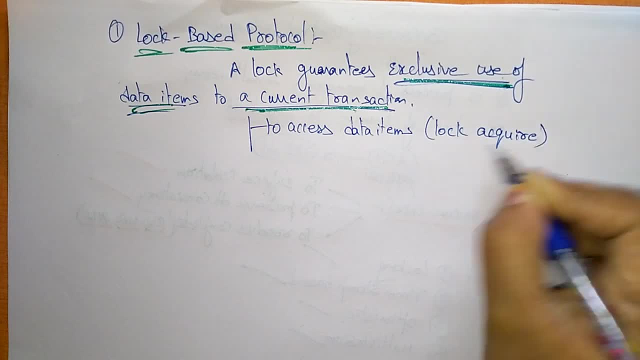 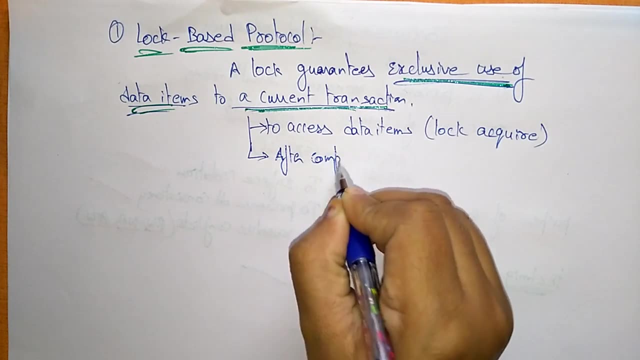 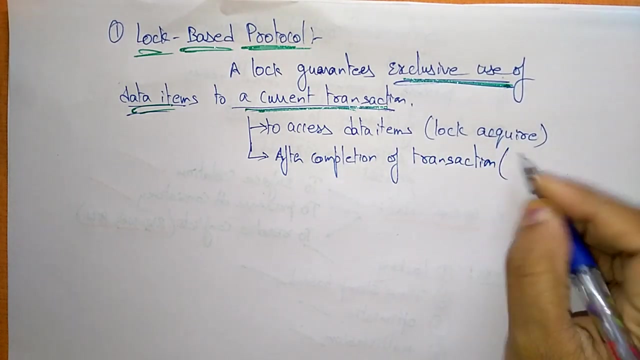 acquire By lock, acquire it, access the data items. So next, what it does after completion: after completion of transaction, it releases the lock. So in the lock based protocol, first the lock will be acquired by the transaction. So once it acquires the transaction, it 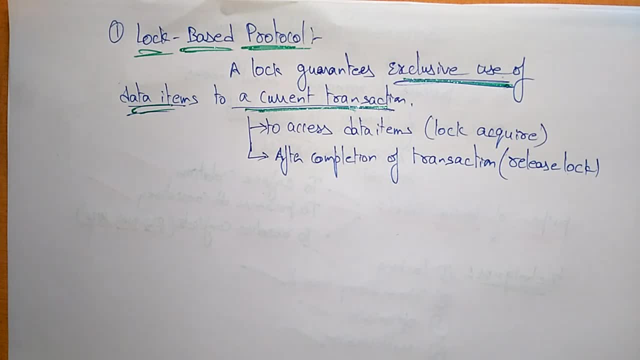 does the operation by accessing the data items After completion transaction. it releases the lock first, acquiresミ lock, after that releases log. Here all data items must be accessed in a mutually exclusive manner. So here different types of lock are singing. Soの number of data items must be access in a mutually exclusive manner. So you, different types of lock. 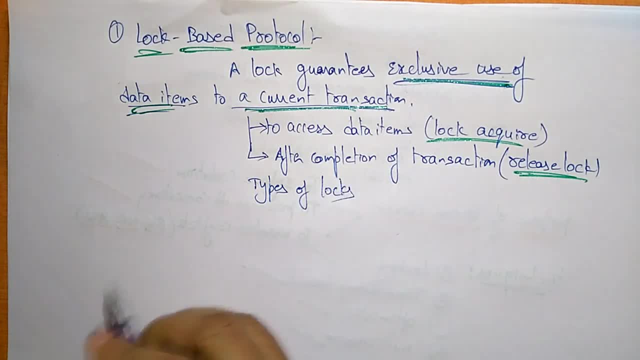 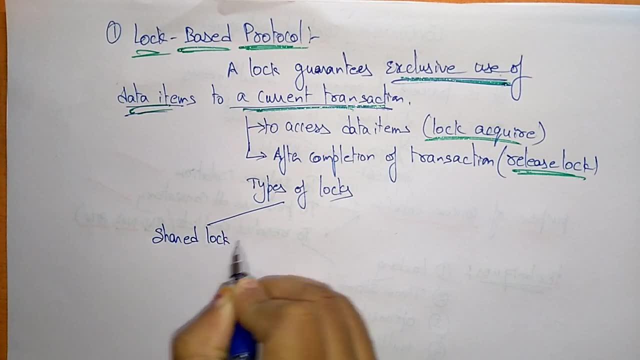 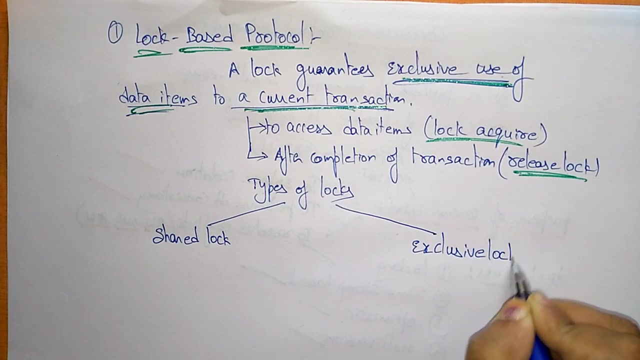 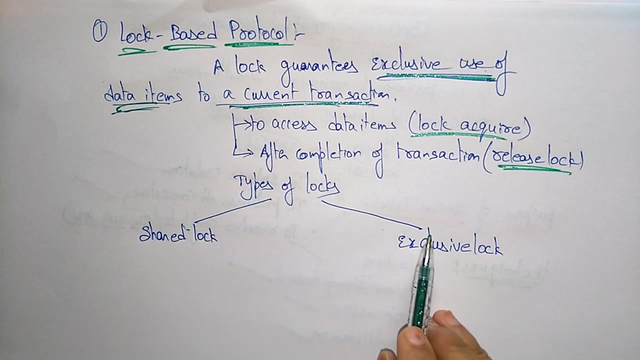 Here all data items must be access in a mutually exclusive manner. So you different types of lock will be there, types of locks. so the two types of locks, or shared lock and exclusive lock. okay, so these are the two different types of locks that are used in the lock based protocol. one is a shared lock and next is the excused lock. 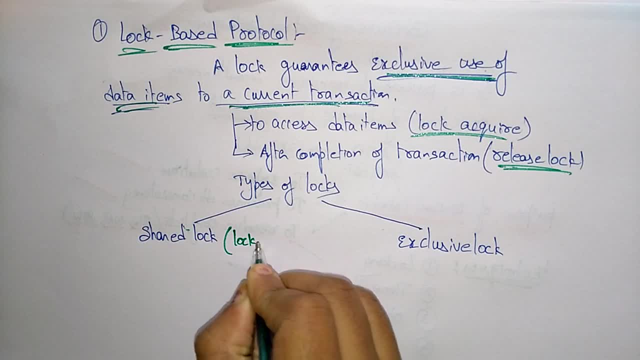 so shared lock will be called as lock s. so whenever it is lock s, you call it as a shared lock, and exclusive lock means lock X. so exclusive lock means lock X is the exclusive lock. so what is a shared lock here? in the shared lock we use only 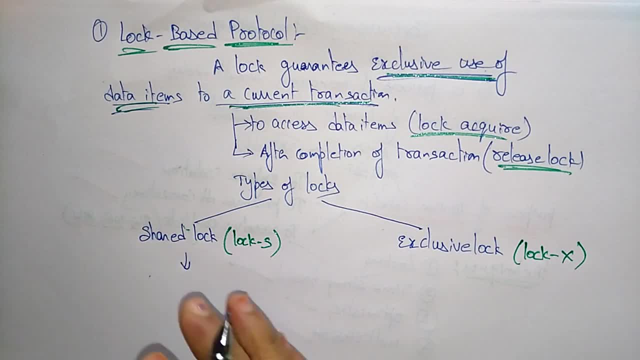 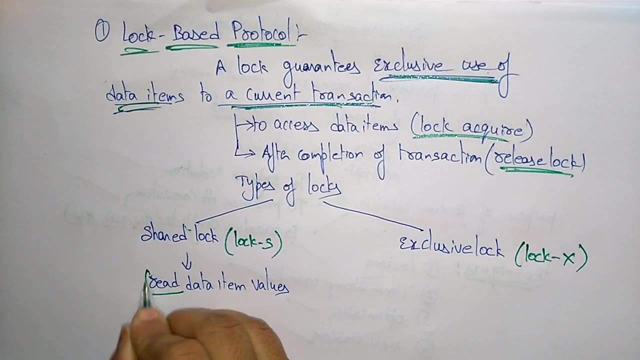 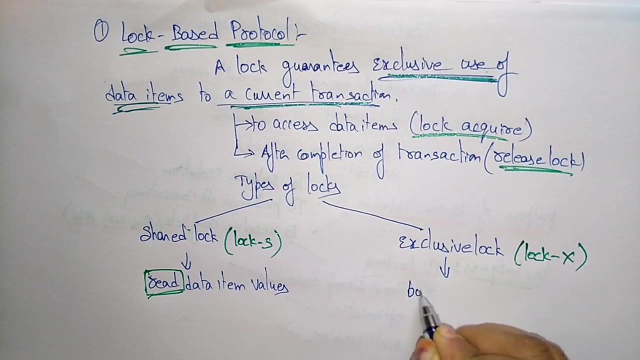 that here in the if the transaction is using the shared lock means this transaction can read only the data items, data item values. so the main purpose of shared lock is it only reads the data items values, whereas- excuse exclusive law- use it for both read and write data. 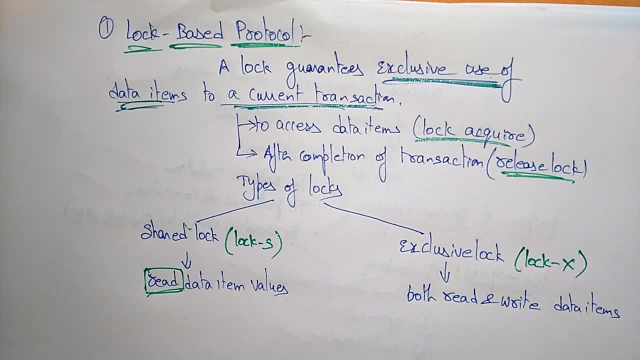 item values. so exclusive log is used for both read and write operations, whereas a Shared lock is only for read. If you want to read the data items, you just use the shared lock If you want to save the data items. if you want to read and save the data items, you just use the exclusive lock. 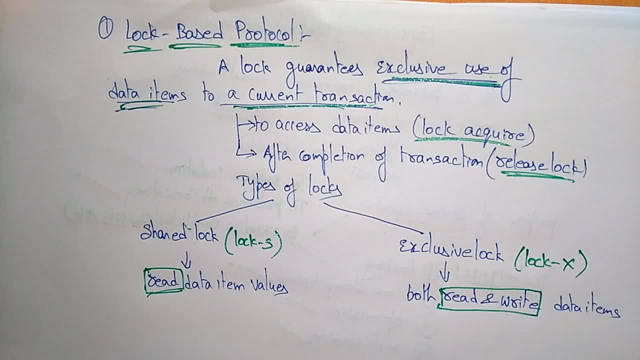 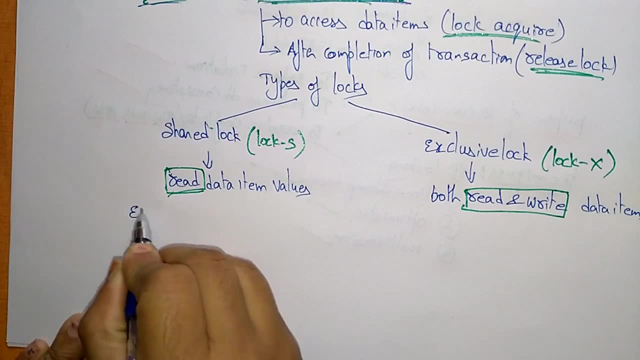 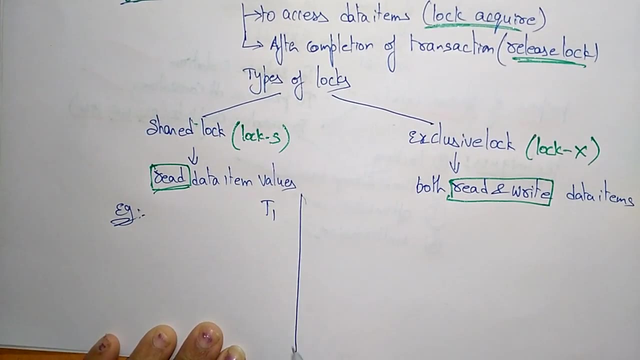 Okay so these are the different types of locks used: shared lock and exclusive lock. So let us see the example how the lock will work. Okay so, example of lock based protocol. Let us take two transactions: T1 and T2.. 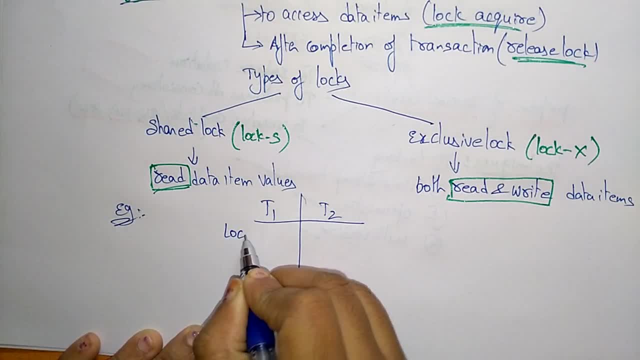 So first what it is doing. first lock, So which lock we are taking? Exclusive lock. So whenever you take, X means you can perform both read and write operations XB. So now the transaction: the data item is locked. Okay, first read B. 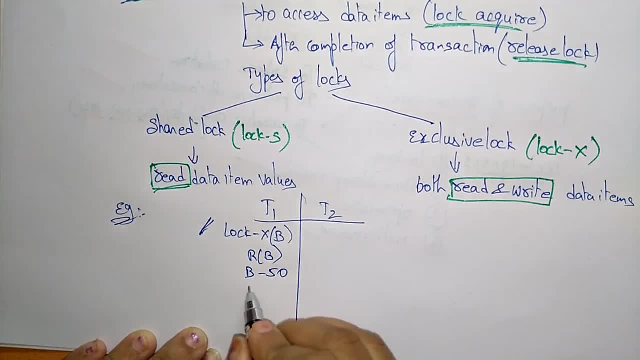 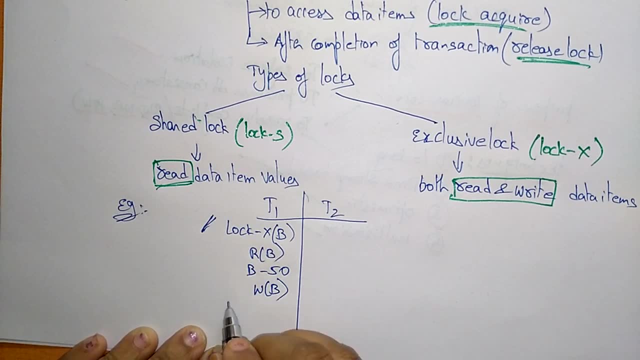 After that B minus some 50. You are doing means you are deducting some 50 amount From the B account And then write B: Okay, now unlock B. So whenever you use unlock B means now the data item is released. 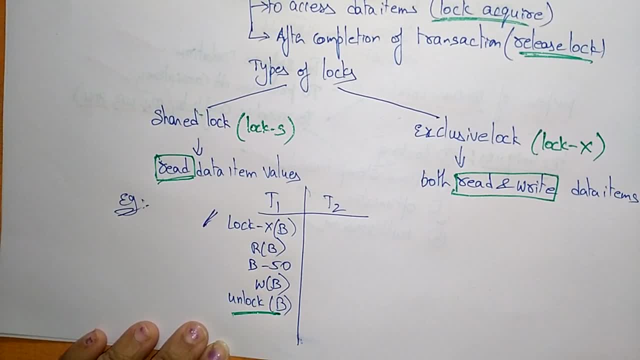 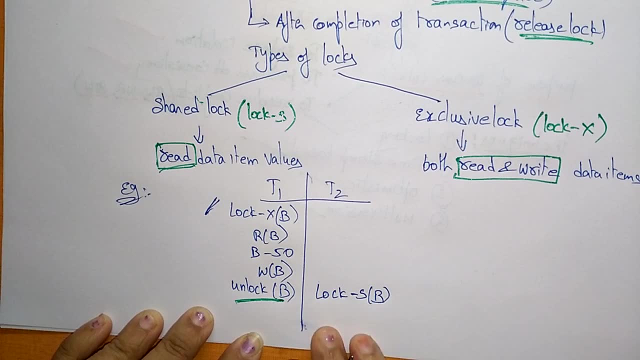 Then this data item can be used by the other transaction. Okay, suppose if you use lock SB, SB means shared lock, So in the shared lock you can only read the data item. So read the B, B value and unlock B. 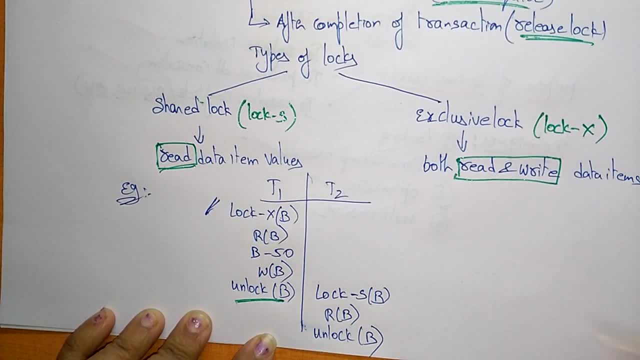 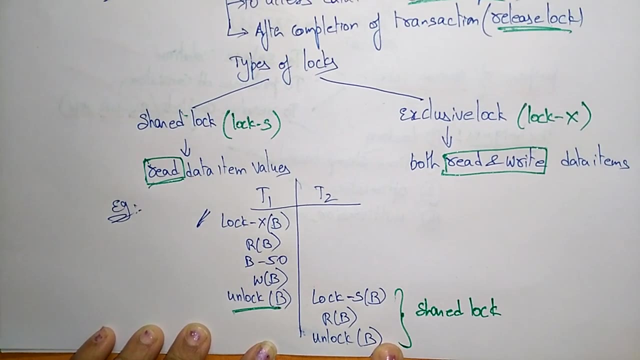 Okay, so this you call it as a shared lock. First you are locking that. acquiring the data items means lock, acquire is there. After that you are reading the operation and you are unlocking the data item. Okay, so this is a shared lock.